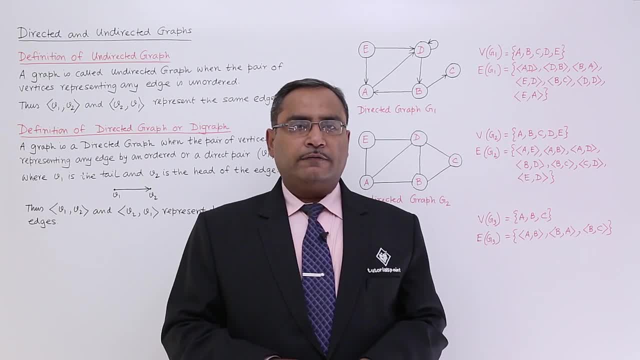 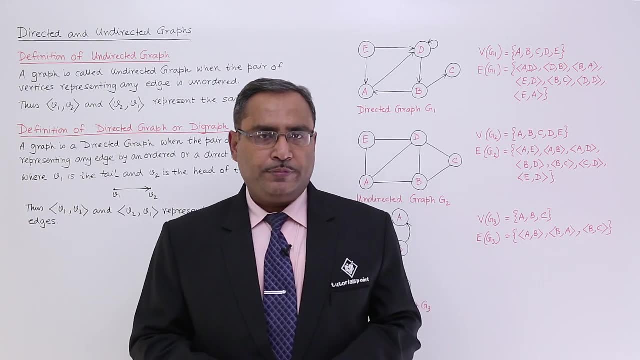 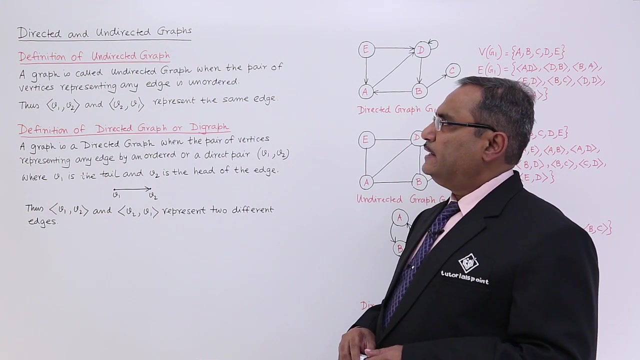 We are discussing directed graph and undirected graph, with the proper definition, with the example to clear our conception. At first we are starting with the undirected graph. So definition of undirected graph. A graph is called undirected graph when the pair of vertices representing 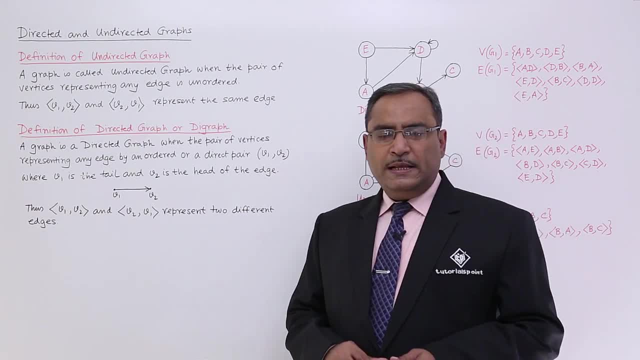 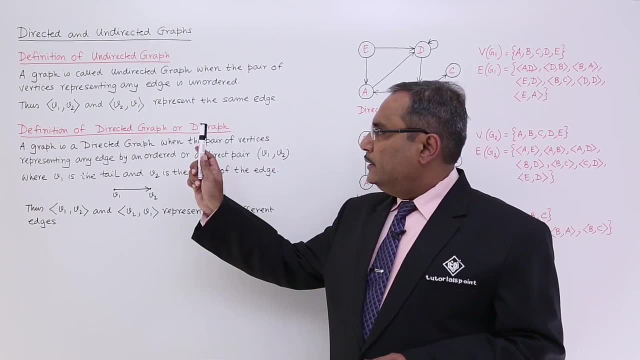 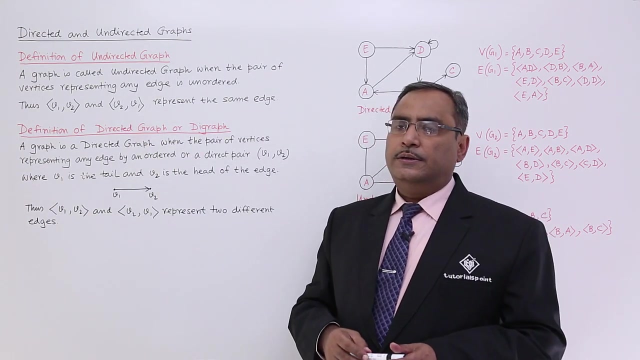 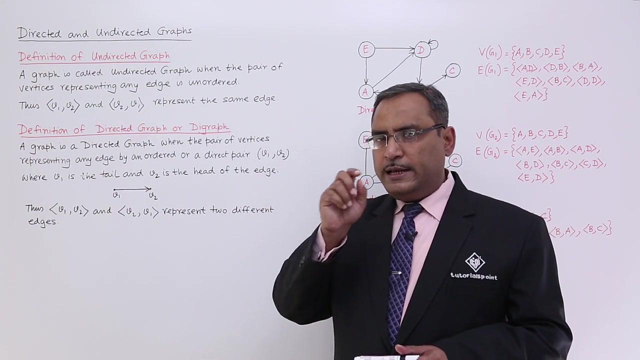 any edge is unordered. That means, let us suppose there is a particular edge which is connecting vertex v1 and v2.. Then v1, v2 and v2, v1: both will represent the same edge and then the graph will be known as the undirected graph. There will be no arrow, There is no conception of any tail, and 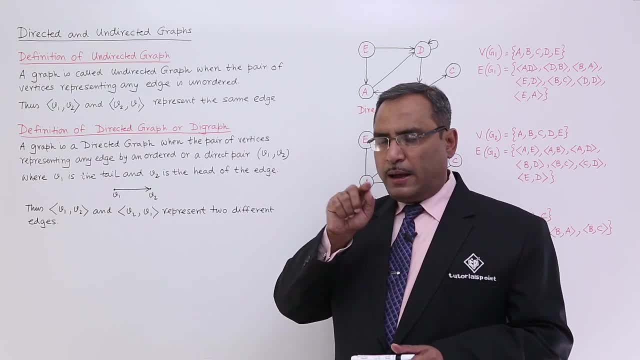 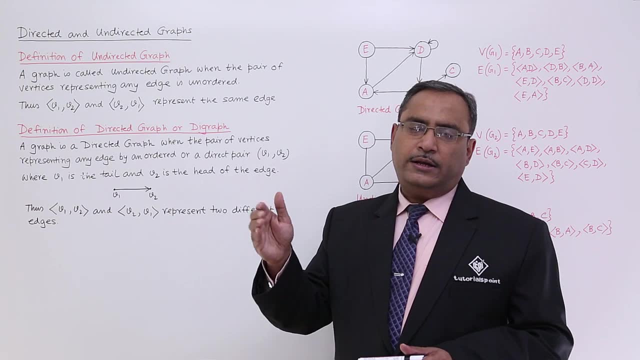 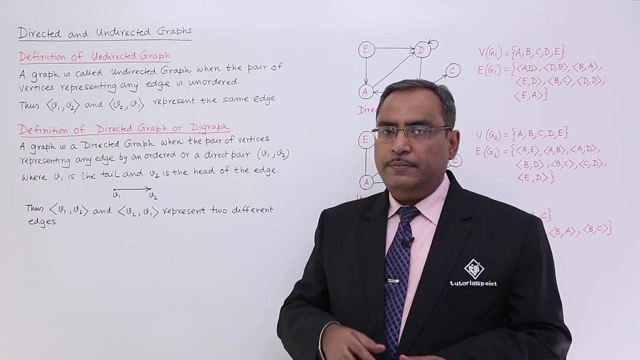 head. So there is no conception. So v1 and v2 have been connected. They have been connected by a single edge. I cannot tell that v1 is the tail or v2 is the head or vice versa. So v1, v2 and v2: v1 will produce and represent the same edge of the graph and 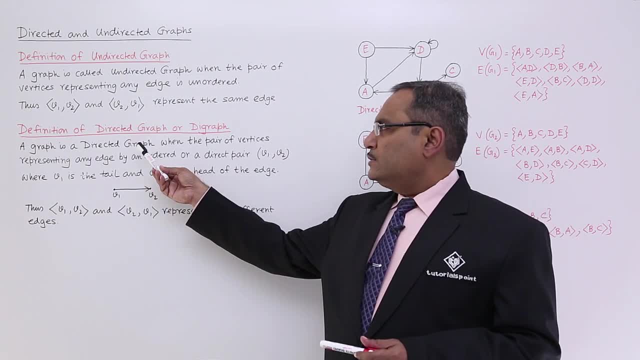 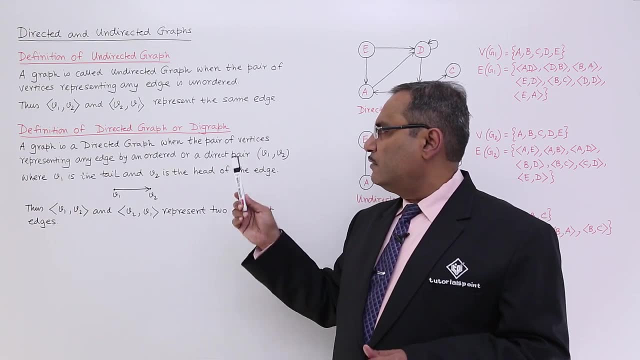 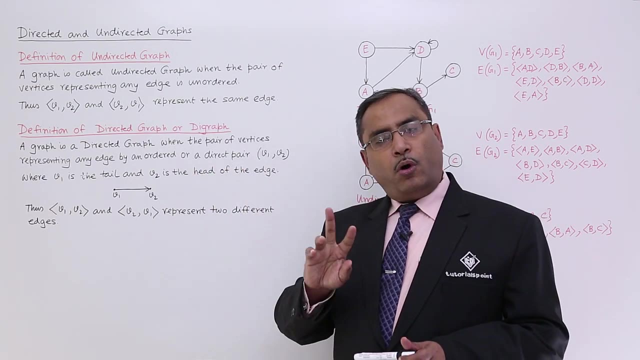 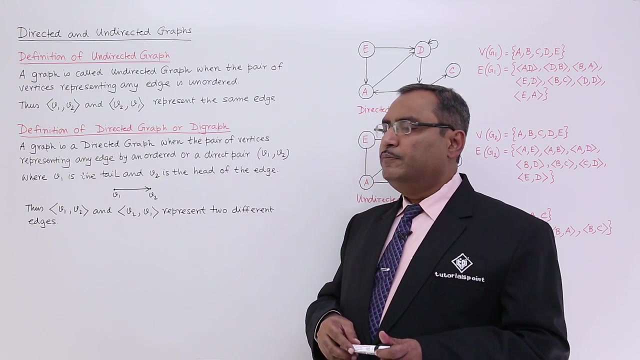 that is why the graph is called undirected In case of directed graph also. in short, it will be called as digraph. A graph is a directed graph when the pair of vertices representing any edge by an ordered Or a direct pair. So ordered pair or direct pair: v1- v2.. Here v1 is the tail and v2 is the head of. 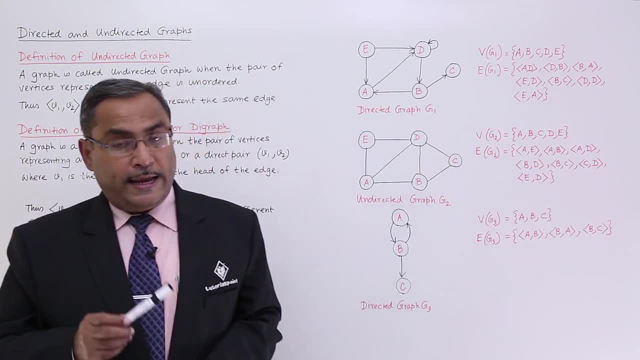 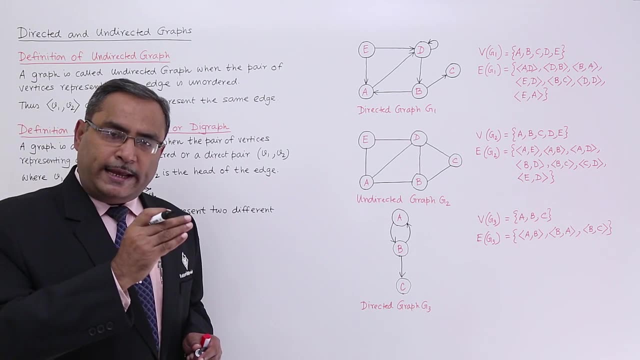 the edge. So v1 is the tail and v2 is the head of the edge. So let us suppose we are having this particular v1 and v2.. So from v1 the edge has been originated and it has got terminated to v2.. 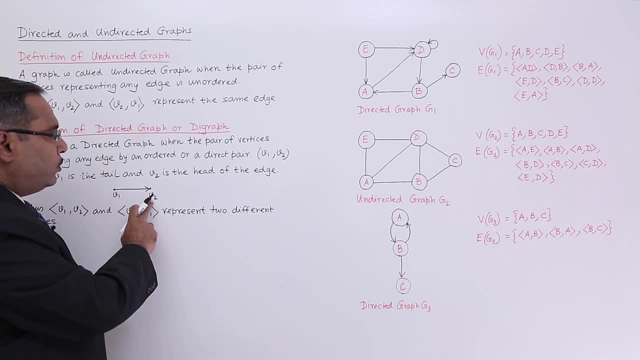 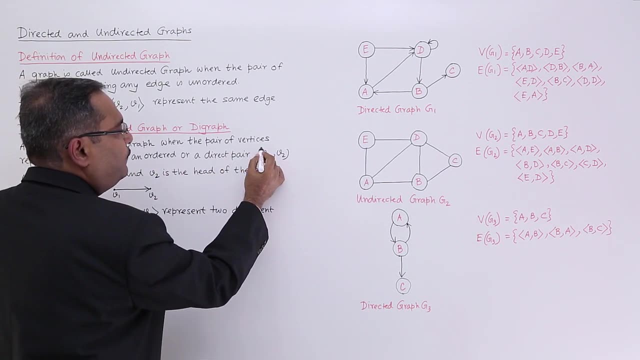 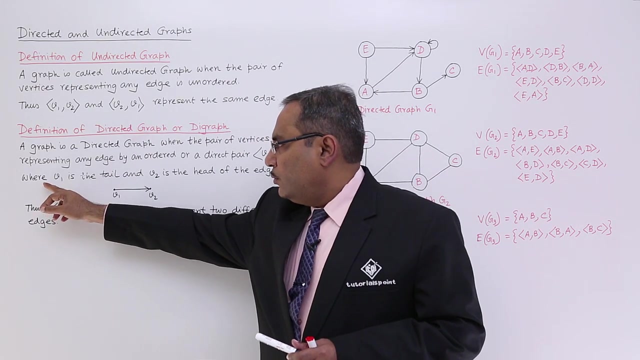 So it will be known as the tail and it will be known as the head. So that is why it is written that any edge by an ordered or a direct pair, v1 and v2.. So in this way I am writing the same, So obviously here where v1 is the tail and v2 is the head of the edge. Thus v1, v2 and v2, v1. 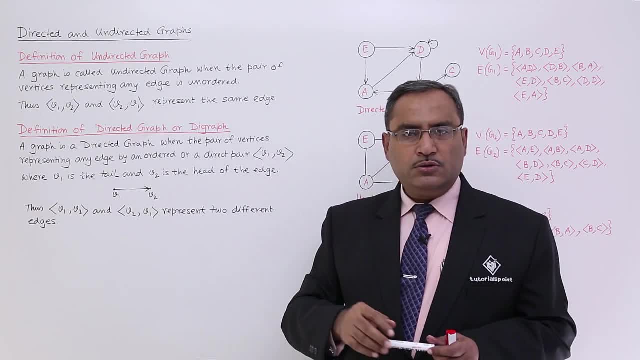 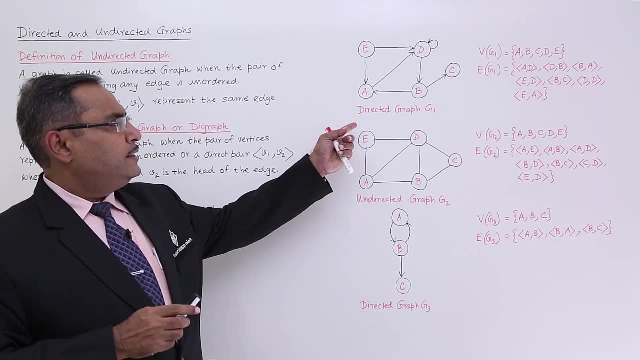 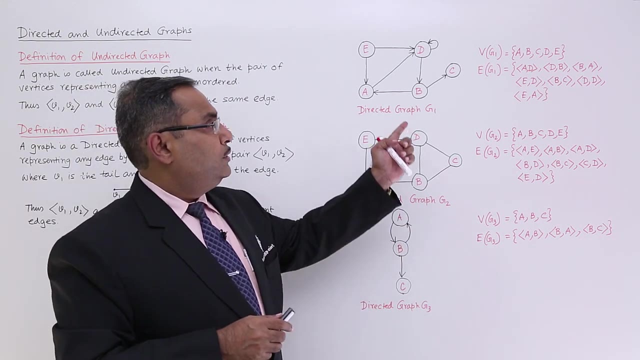 represent two different edges. So let us go one example, one or two examples with the help of which we can explain. So this is the graph Here. you see, this is the directed graph. This is undirected. there is no arrows are there, and this is also, again, a directed graph. So this graph consists: